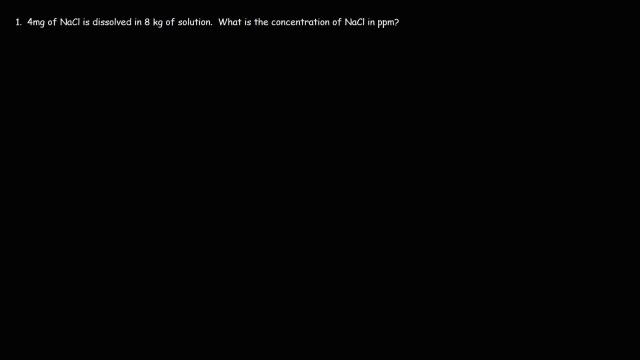 In this video, we're going to work on solving problems associated with units of concentration such as ppm and ppb. ppm stands for parts per million. ppb stands for parts per billion. In order to calculate the concentration in ppm, you need to take the mass of the solute in grams. 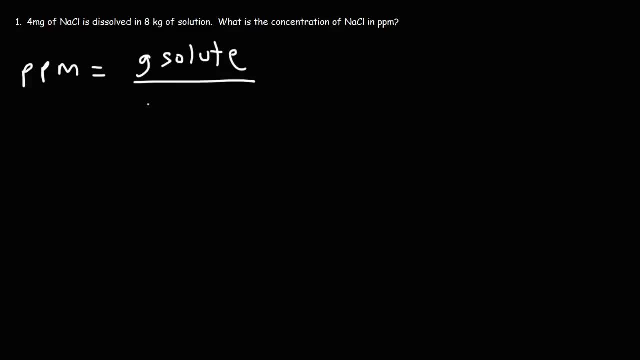 and divide it by the mass of the solution in grams and then multiply that by 10 to the 6.. ppm is a special type of concentration. It is used for substances with a very low concentration in solution. Now, there are many different forms of concentration. Perhaps you heard of 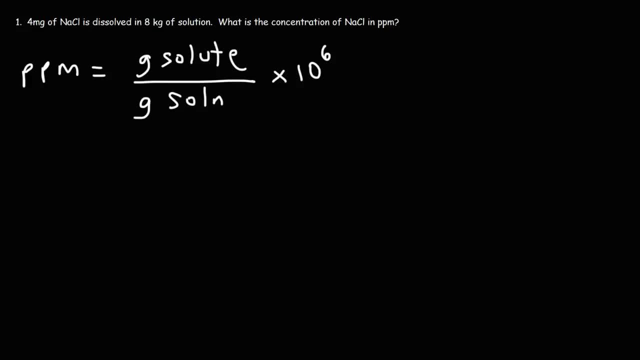 molarity, molality normality, mass percent, volume percent- All of these are used to calculate the concentration. in ppm You can use to represent the concentration of a solution, But in this video we're going to focus on ppm and ppb. 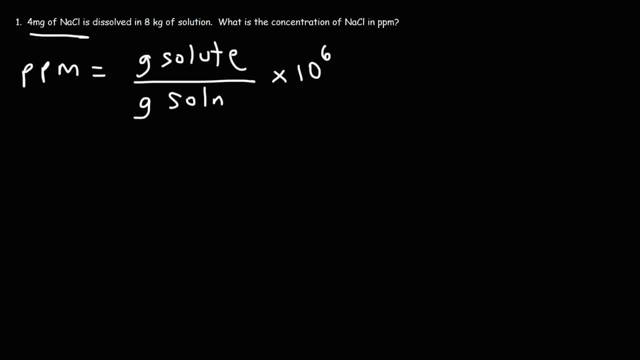 Now in this example problem we have four milligrams of sodium chloride. We need to convert that to grams. One gram is equal to a thousand milligrams. So to convert from milligrams to grams, divide by a thousand. So four divided by a thousand. 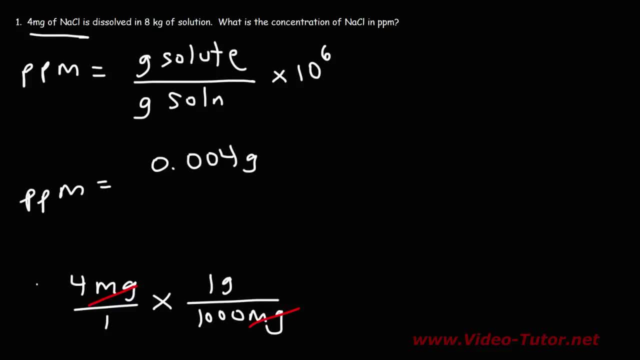 is 0.04.. So that's how much grams of solute we have in this solution. And now we have eight kilograms of solution. To convert kilograms to grams, you need to multiply by a thousand. One kilogram is equal to a thousand grams. 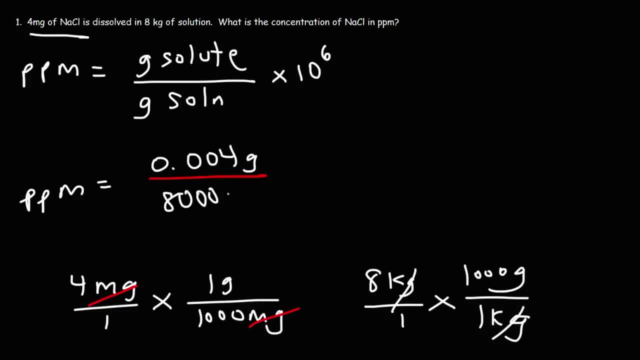 So eight kilograms is a thousand grams, And then we're going to multiply this by 10 to the 6., So 0.04.. Divided by a thousand and then times one, times 10 to the 6., This is 0.5.. So this is the. 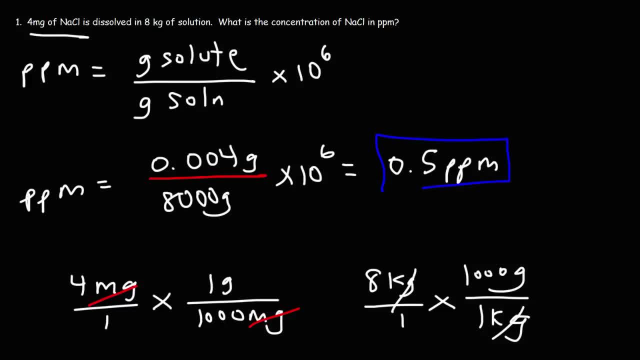 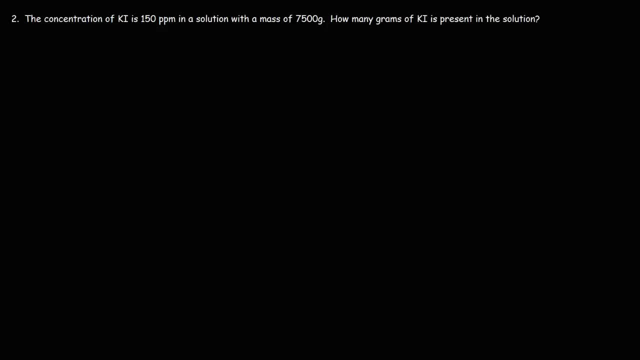 concentration of sodium chloride in the solution. It's 0.5 parts per million. Now let's move on to the next problem. The concentration of potassium iodide is 150 parts per million in a solution with a mass of 7,500 grams. How many grams of Ki? 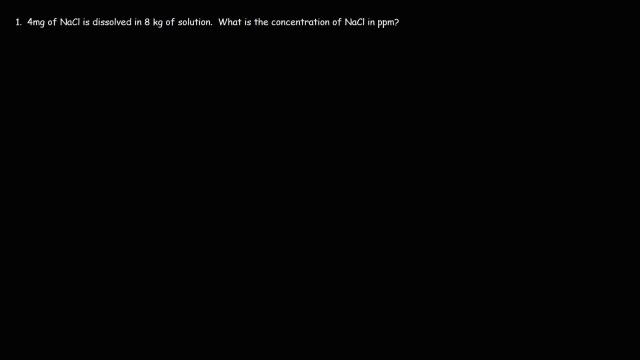 In this video, we're going to work on solving problems associated with units of concentration such as ppm and ppb. ppm stands for parts per million. ppb stands for parts per billion. In order to calculate the concentration in ppm, you need to take the mass of the solute in grams. 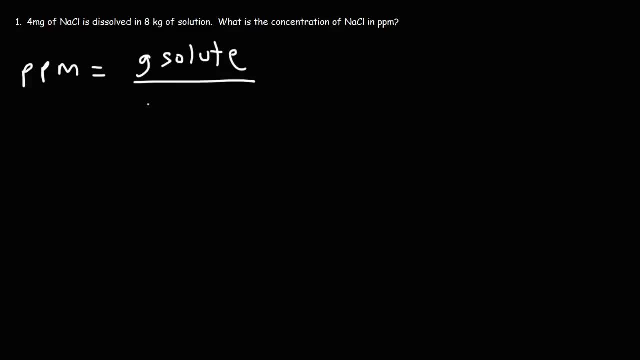 and divide it by the mass of the solution in grams and then multiply that by 10 to the 6.. ppm is a special type of concentration. It is used for substances with a very low concentration in solution. Now, there are many different forms of concentration. Perhaps you heard of 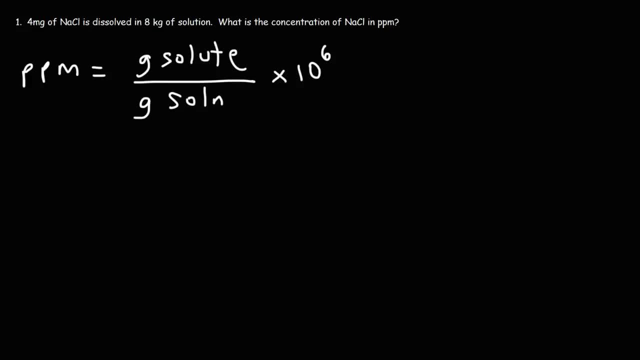 molarity, molality normality, mass percent, volume percent- All of these are used to calculate the concentration. in ppm You can use to represent the concentration of a solution, But in this video we're going to focus on ppm and ppb. 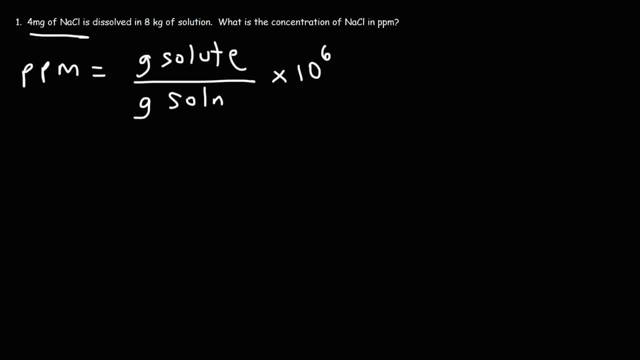 Now in this example problem we have four milligrams of sodium chloride. We need to convert that to grams. One gram is equal to a thousand milligrams. So to convert from milligrams to grams, divide by a thousand. So four divided by a thousand. 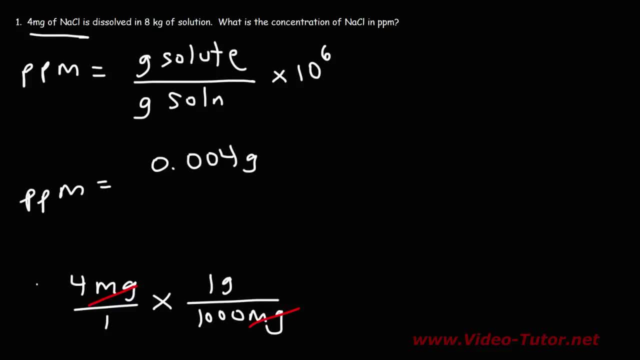 is 0.04.. So that's how much grams of solute we have in this solution. And now we have eight kilograms of solution. To convert kilograms to grams, you need to multiply by a thousand. One kilogram is equal to a thousand grams. 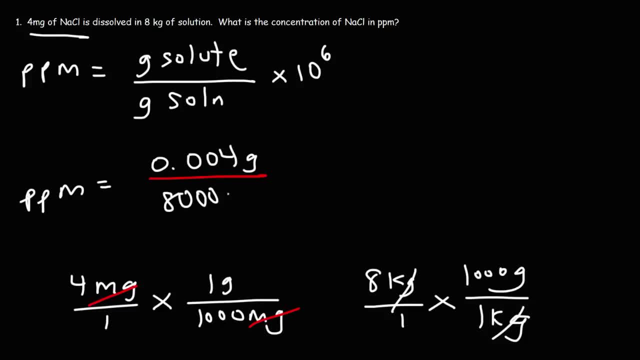 So eight kilograms is a thousand grams, And then we're going to multiply this by 10 to the 6.. So 0.04 is equal to a thousand grams, And then we're going to multiply this by 10 to the 6.. 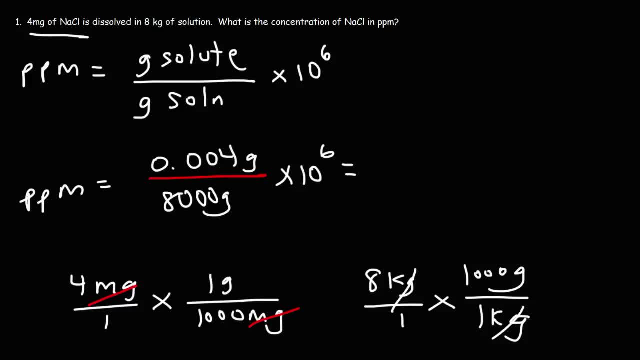 So 0.04 divided by 8,000.. And then times one times 10 to the 6. This is 0.5.. So this is the concentration of sodium chloride in a solution. It's 0.5 parts per million. 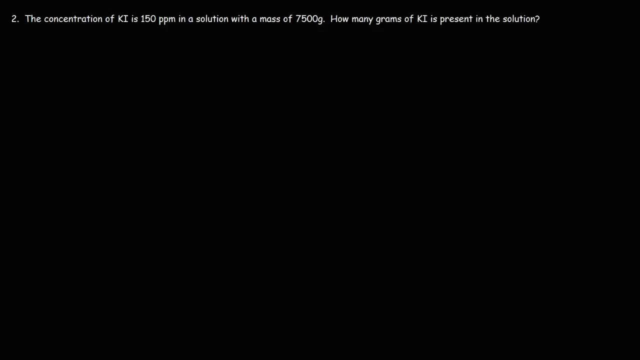 Now let's move on to the next problem. The concentration of potassium iodide is 150 parts per million in a solution with a mass of 7,500 grams. How many grams of Ki is present in the solution? Now? it's helpful to represent the concentration in ppm in. 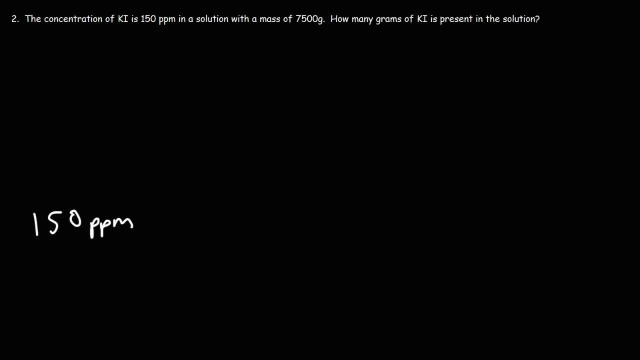 terms of the grams of solute relative to the grams of solution. So 150 ppm means that there's 150 grams of potassium for every 10 to the 6 grams of solution, And Expressing the ppm concentration in this way will make it easier for us to solve the problem using unit conversion. 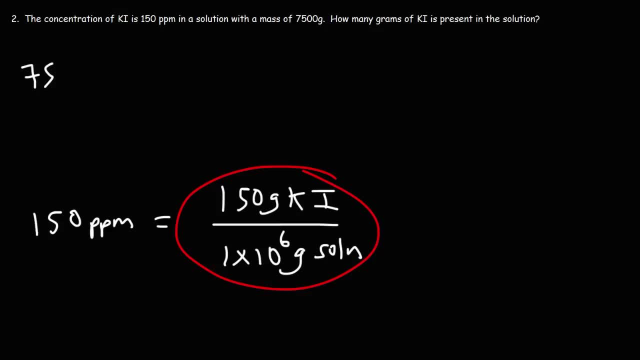 So let's begin. Let's start with the mass that we're given, That is, 7,500 grams of solution, And now let's convert this to the grams of Ki. So, using this concentration, we know that there's 150 grams of potassium iodide. 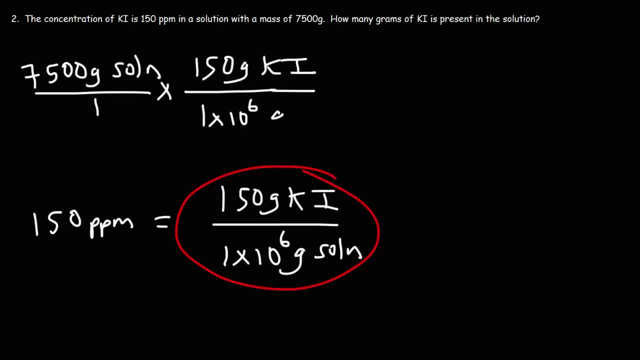 for every 1 million grams And that is the mass of the solution. So in this example we can see that the unit grams of solution cancels. so it's going to be 7,500 times 150, divided by 1 times 10 to the 6.. 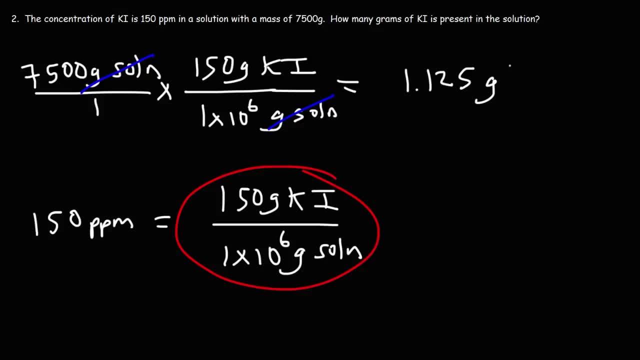 So the answer is 1.125 grams of potassium iodide. So that's how you can calculate the mass of the solute, given the solution concentration in ppm. Now let's confirm that this answer is correct. So let's recalculate our ppm concentration. 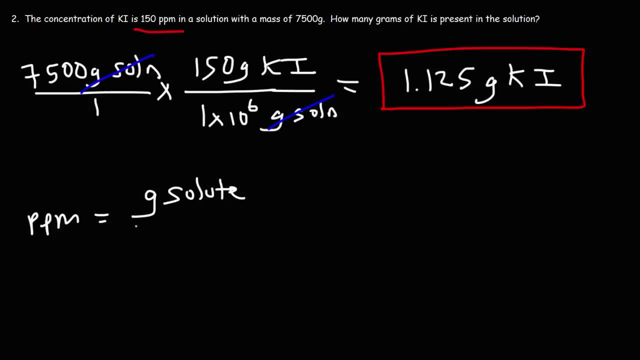 So we know that it's the mass of solute in grams divided by the mass of the solution in grams, times 10 to the 6. The grams of solute is what we just got, That's 1.125 grams of Ki. The grams of solution is 7500 grams. 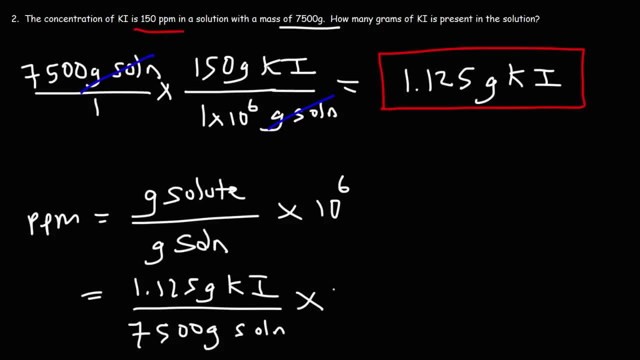 And then we're going to multiply that by 10 to the 6. If our answer is correct, we should get 150. That is, we should get this number, So 1.125 divided by 7500 times 1 times 10 to the 6. 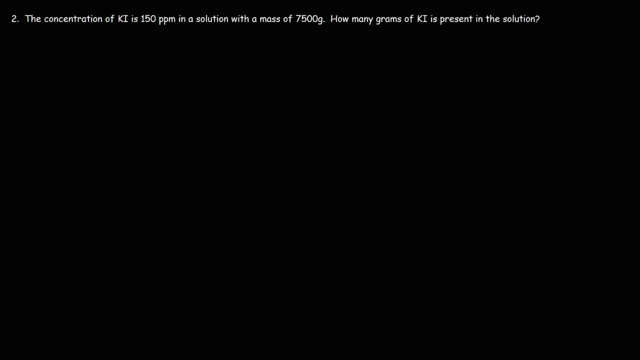 is present in the solution. Now it's helpful to represent the concentration in ppm in terms of the grams of solute relative to the grams of solution. So 150 ppm means that there's 150 grams of potassium for every 10 to the 6 grams of solution. 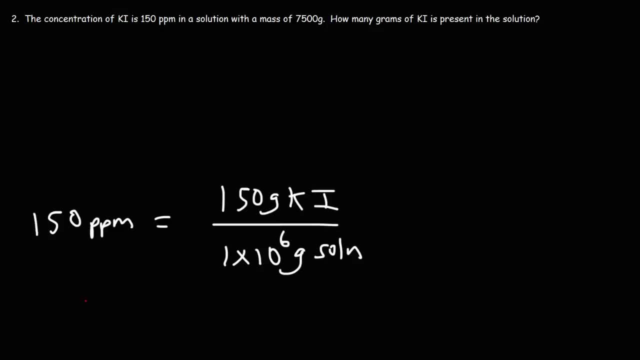 And expressing the ppm concentration in this way will make it easier for us to solve the problem using unit conversion. So let's begin. Let's start with the mass that we're given, That is, 7,500 grams of solution, And now let's convert this to the grams of Ki. 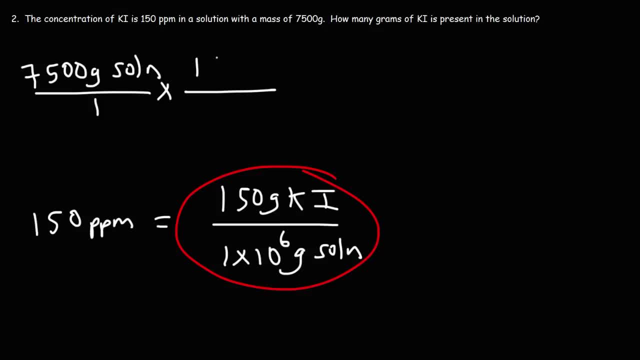 So using this concentration, we know that there's 150 grams of potassium iodide For every 1,000,000 grams of solution. So in this example we can see that the unit grams of solution cancels, So it's going to. 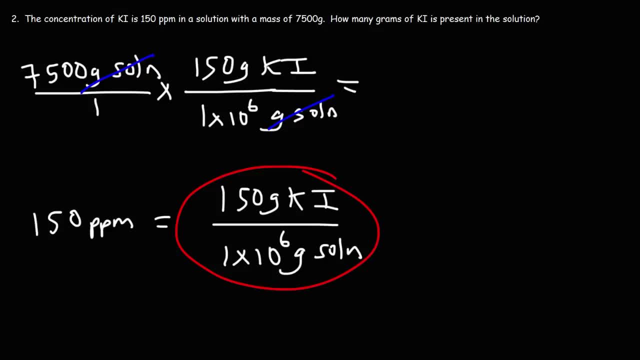 be 7,500 times 150, divided by 1 times 10 to the 6.. So the answer is 1.125 grams of potassium iodide. So that's how you can calculate the mass of the solute, given the solution concentration. 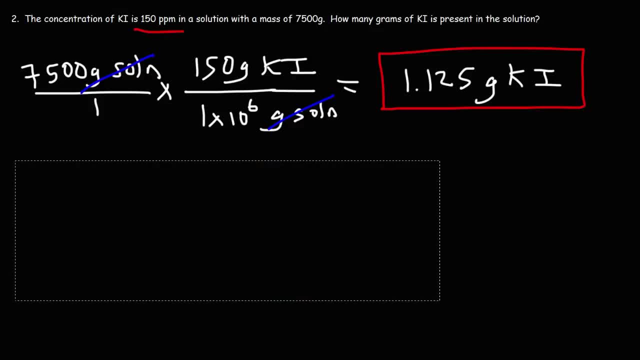 in ppm. Now let's confirm that this answer is correct. So let's recalculate our ppm concentration. So we know that it's the mass of solute in grams divided by the mass of the solution in grams, times 10 to the 6.. 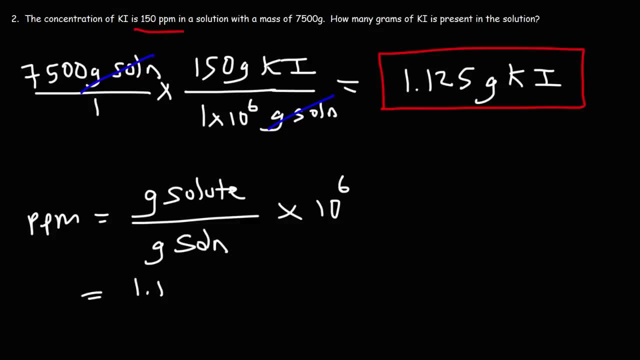 The grams of solute is what we just got, That's 1.125 grams of Ki. The grams of solution is 7,500 grams, And then we're going to multiply that by 10 to the 6. If our answer is correct, we should get 150.. That is, we should get this number. 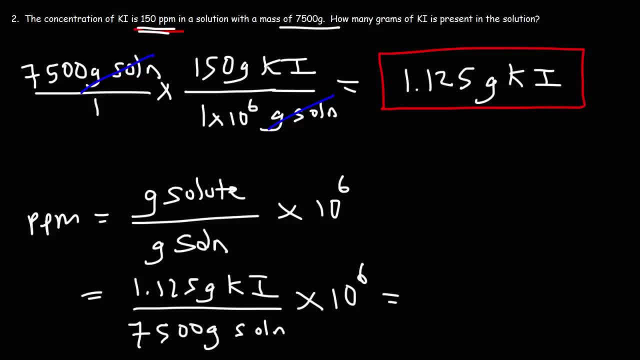 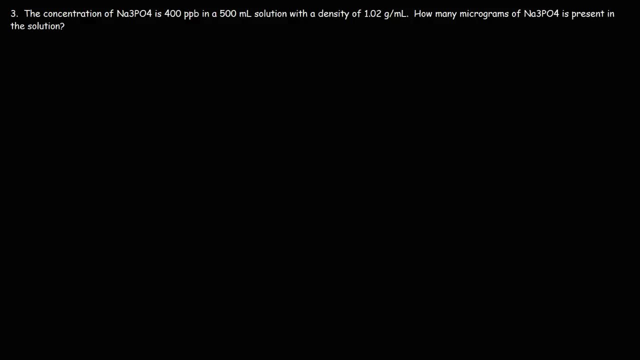 So 1.125 divided by 7,500 times 1 times 10 to the 6 is indeed 150 ppm. So this helps us to see that the answer that we have here is indeed correct. Now let's move on to the next problem: The concentration of sodium. 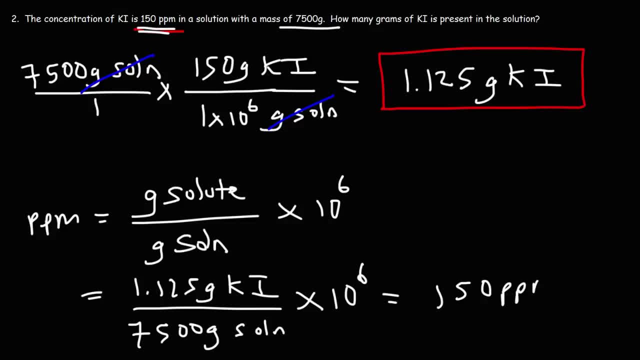 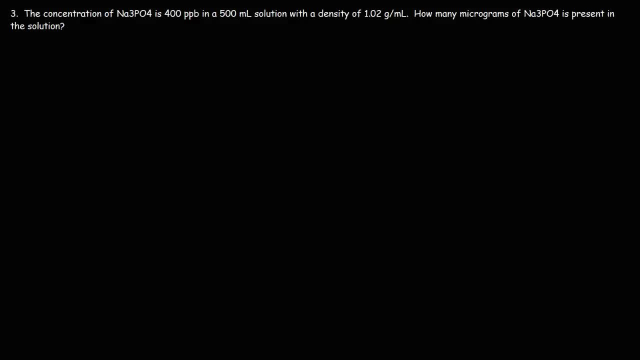 is indeed 150 ppm, So this helps us to see that the answer that we have here is indeed correct. Now let's move on to the next problem. The concentration of solute sodium phosphate, Na3PO4, is 400 parts per billion in a 500 mL solution. 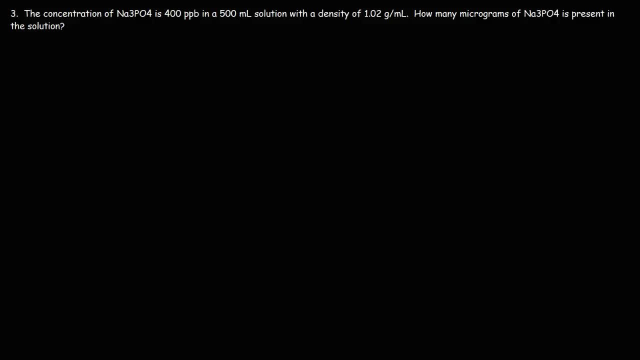 with a density of 1.02 grams per mL. How many micrograms of sodium phosphate is present in this solution? Now, for those of you who want to try this problem, feel free to pause the video and then, when you're done, play it to see if you have the right answer. 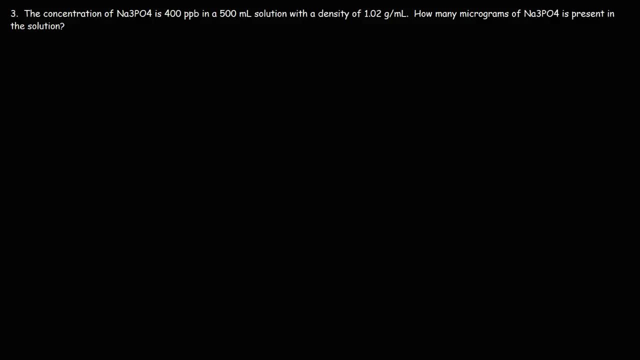 So let's begin. Let's start with the mass of sodium phosphate. Now notice that we're given the volume of the solution and the density. Combining these two things can give us the mass of the solution. So we have a volume of 500 mL. Now we're going to multiply that by the density of the solution. 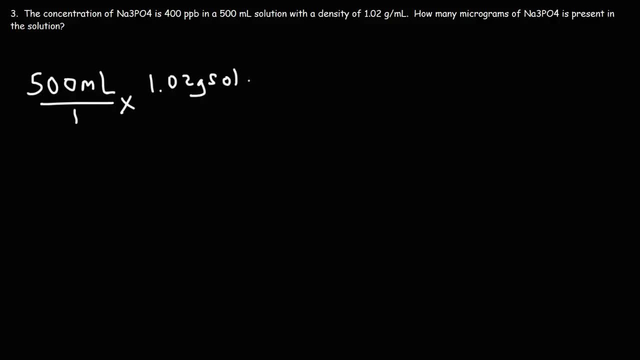 There's 1.02 grams of solution per 1 mL. That's what the density tells us, And so we could cancel the volume, That is, the units of mL, And this will give us the grams of the solution. Now, the solution concentration is 400 parts per billion. 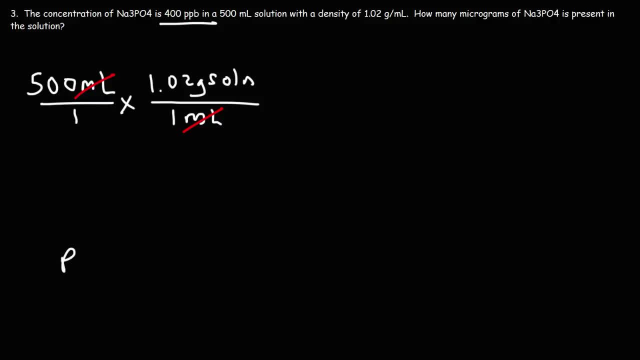 The formula for parts per billion is grams of solute divided by the grams of solution, But the only difference is, instead of multiplying it by a million or 10 to the sixth, we are going to multiply it by a billion or 10 to the ninth. So that's the formula for. 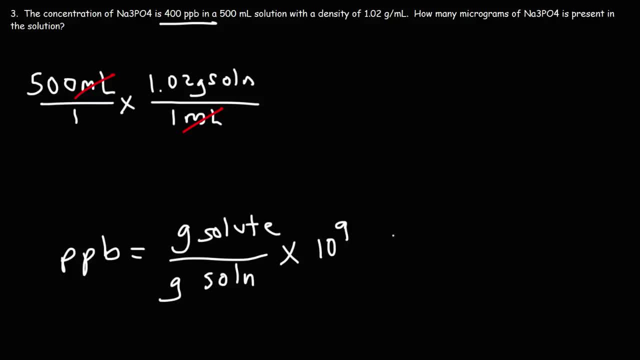 the parts per billion concentration. Now, in this example, we have 400 parts per billion. We want to express this as the ratio of grams of solute to grams of solution. Now, this means that we have 400 grams of solute, the solute being Na3PO4. 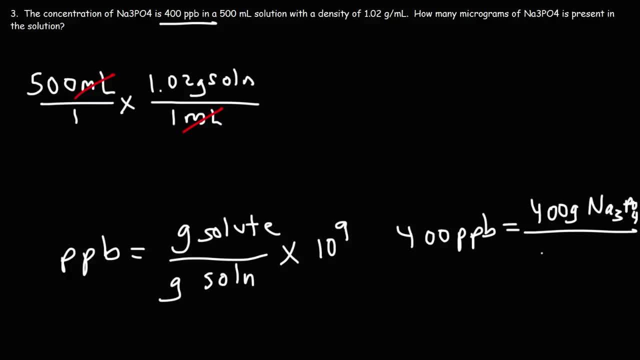 divided by a billion grams of solution, or one times 10 to the ninth grams of solution. So, since we're dealing with unit conversion, we want to express 400 parts per billion in this format. So that's what we're going to write in the next fraction. 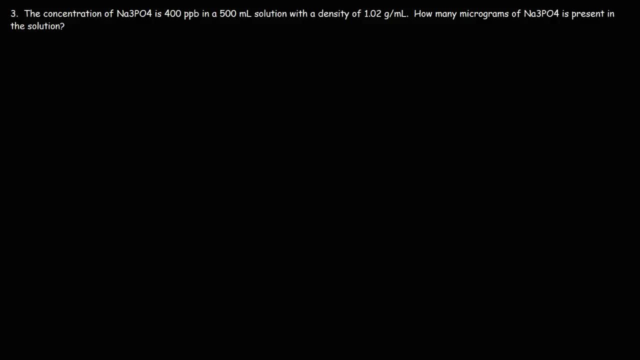 Sodium phosphate, Na3PO4, is 400 parts per billion in a 500 mL solution with a density of 1.02 grams per mL. How many micrograms of sodium phosphate is present in this solution? Now, for those of you who want to try this problem, feel free to pause the video and 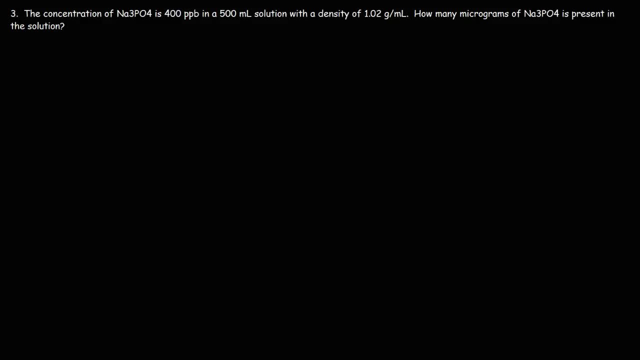 then, when you're done, play it to see if you have the right answer. So let's begin. Let's start with the mass of the solution. Now notice that we're given the volume of the solution and the density. Combining these two things can give us the mass of the solution. 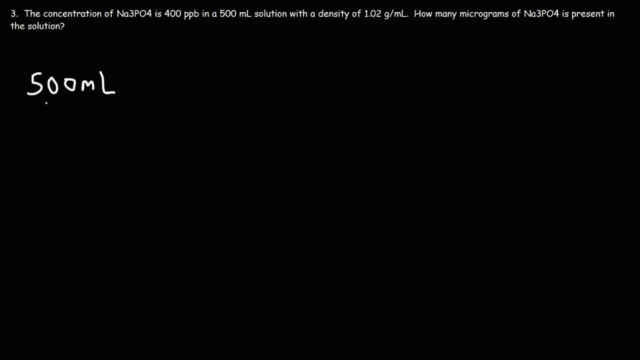 So we have a volume of 500 mL, and we're going to multiply that by the density of the solution, There's 1.02 grams of solution per 1 mL. That's what the density tells us, And so we could cancel the volume. 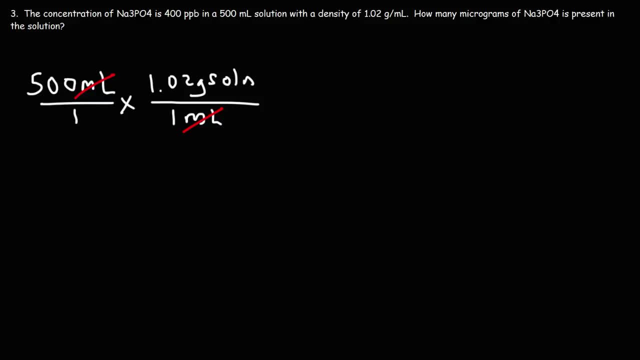 That is, the units of mL, And this will give us the grams of the solution. Now the solution concentration is 400 parts per billion. The formula for parts per billion is grams of solute divided by the grams of solution, But the only difference is, instead of multiplying it by a million or 10, to the 6, we are going. 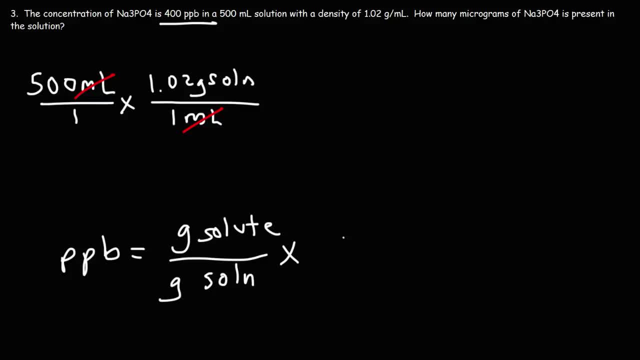 to multiply it by 1.02.. So that's the formula for the parts per billion concentration. Now in this example we have 400 parts per billion. We want to express this as the ratio of grams of solute to grams of solution. 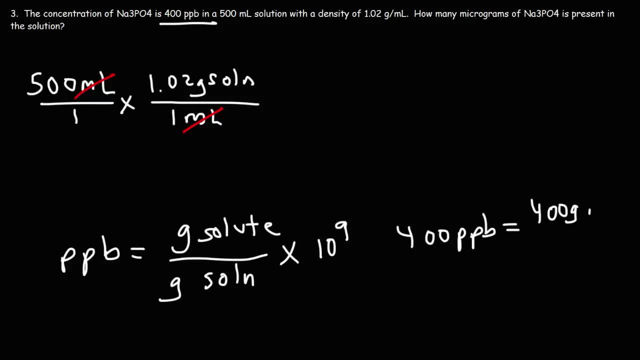 Now this means that we have 400 grams of solute- the solute being Na3PO4, divided by 1.02 grams of solute. So we're going to multiply that by 1.02 grams of solute, or 1 times 10, to the 9 grams of. 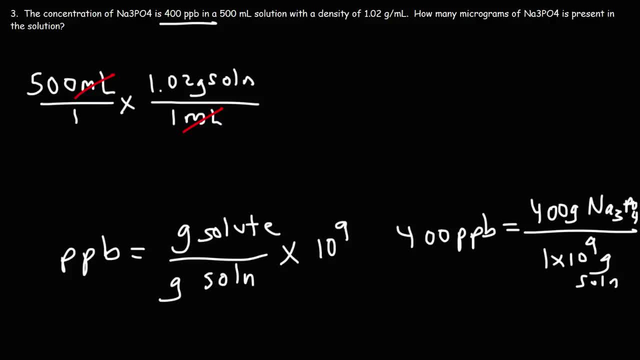 solute. So, since we're dealing with unit conversion, we want to express 400 parts per billion in this format. So that's what we're going to write in the next fraction. So let's write 400 grams of Na3PO4 on the top of the fraction. 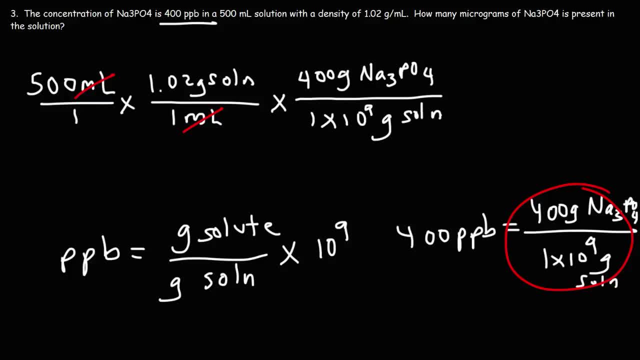 And then 1 times 10 to the 9 grams of solute, And then 1 times 10 to the 9 grams of solute on the bottom. So now we can cross out the grams of solution. Now the last thing we need to do is convert the grams of sodium phosphate to the micrograms. 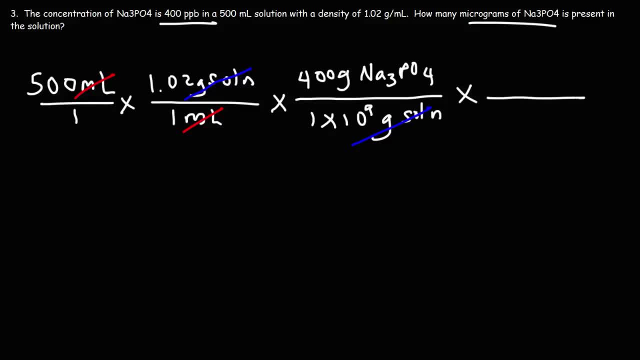 of sodium phosphate. So what's the conversion factor between grams and micrograms? Micro is 10 to the minus 6.. So 1 microgram, 1 microgram, is equal to 10 to the minus 6 grams. So we're going to put 10 to the minus 6 grams on the bottom. 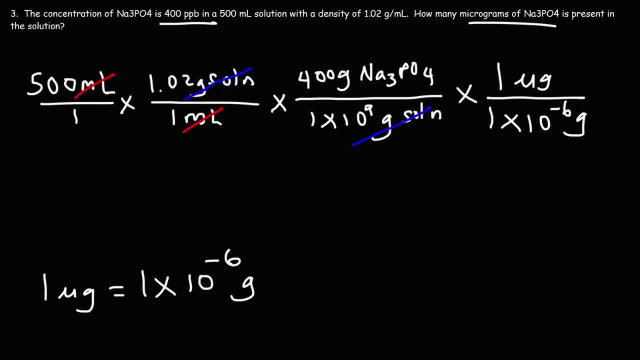 And then we're going to put 1 microgram on top So that we can cross those units. So now let's do the math. If we multiply 500 by 1.02, this will give us the grams of the solution. 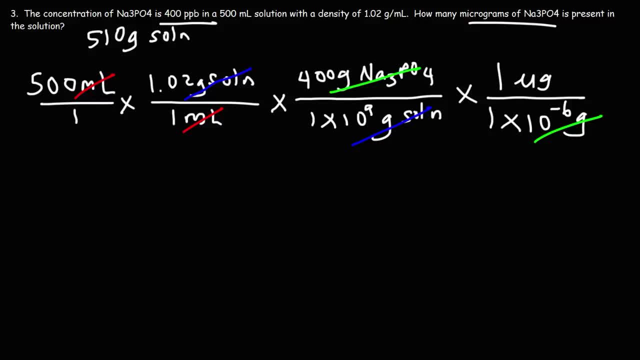 So this is 510 by 1.02.. This is 10 grams of solution. If we take that, multiply it by 400, and divide it by 1 times 10 to the 9,, you'll get 2.04. 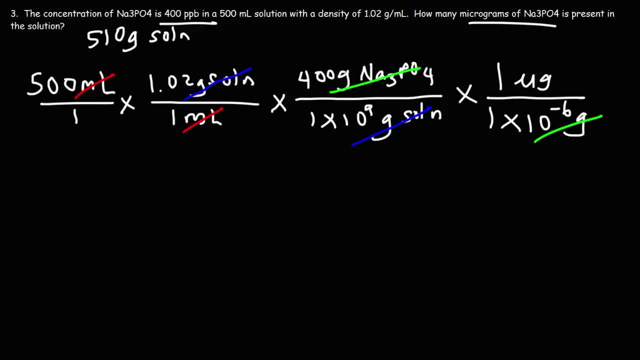 times 10 to the negative 4.. Take that number, divide it by 1 times 10 to the minus 6, and this will give us our answer: 204 micrograms. So that's the mass of sodium phosphate that is present in this solution. 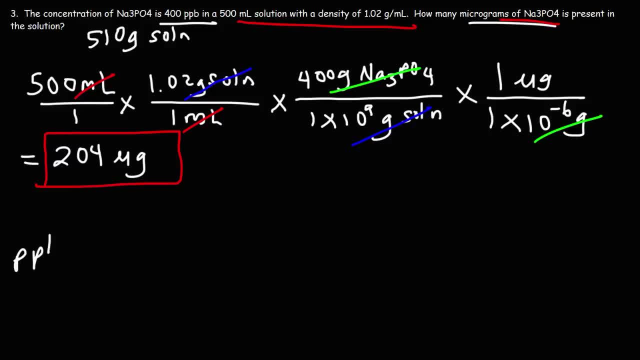 Now, let's go ahead and do the math. Let's go ahead and do the math. Let's confirm our results. The ppb concentration, as mentioned before, is the grams of solute divided by the grams of solution, but times a billion, or 10 to the 9.. 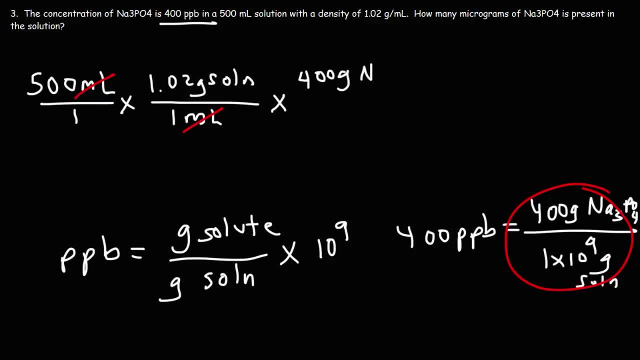 So let's write 400 grams of Na3PO4 on the top of the fraction and then 1 times 10 to the ninth grams of solution on the bottom. So now we can cross out the grams of solution. Now the last thing we need to do. 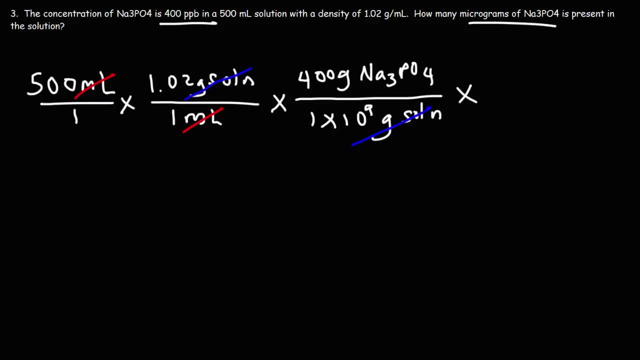 is convert the grams of sodium phosphate to the micrograms of sodium phosphate. So what's the conversion factor between grams and micrograms? Micro is 10 to the minus six. So one microgram is equal to 10 to the minus six grams. So we're going to put 10 to the minus six. 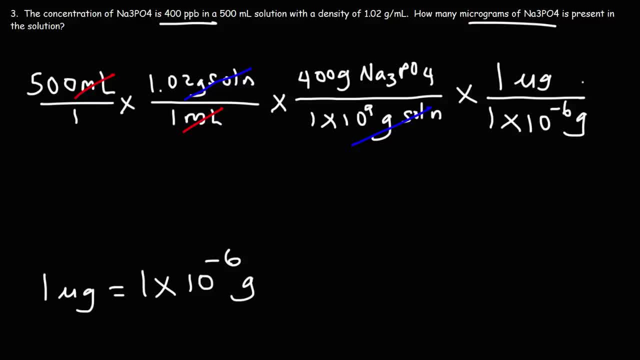 grams on the bottom, and then we're going to put one microgram on top so that we can cross those units. So now let's do the math. If we multiply 500 by 1.02, this will give us the grams of solution. This is 510. 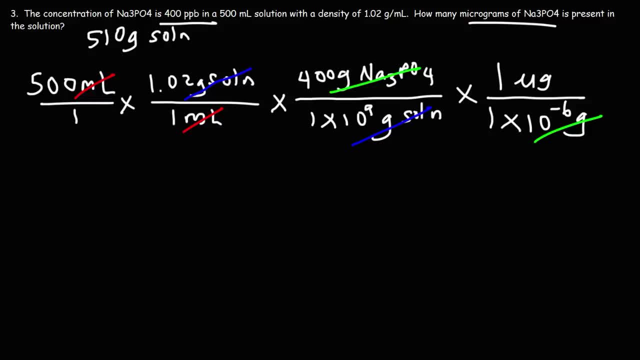 grams of solution. If we take that, multiply it by 400 and divide it by 1 times 10 to the ninth, you'll get 2.04 times 10 to the negative four. Take that number, divide it by 1 times 10 to the minus six. 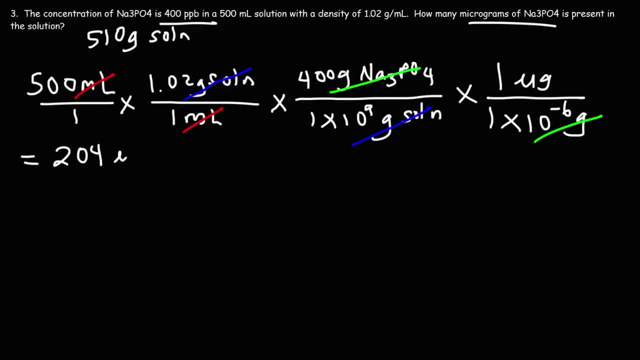 and this will give us our answer: 204 micrograms. So that's the mass of sodium phosphate that is present in this solution. Now let's confirm our results. The PPB concentration, as mentioned before, is the grams of solute divided by the grams of solution, but times a billion, or 10 to the nine. 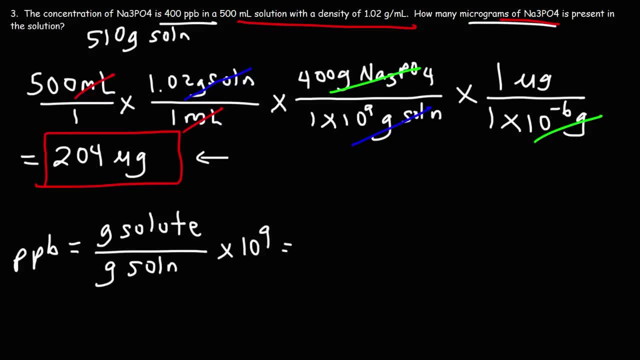 So in this example, the grams of solute is. well, this is the micrograms. So the grams of solute is going to be 204 micrograms, or 204 times 10 to the minus six grams. The grams of solution is what we have here, it's 510. 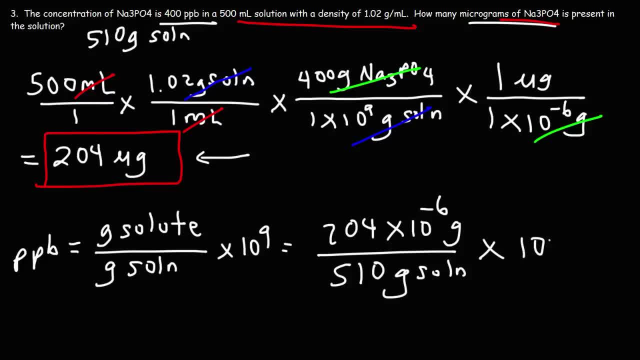 grams of solution, and then let's multiply that by 10 to the nine. If our answer is correct, we should get 400 parts per billion, So 204 times 10 to the minus six, divided by 510 times 1 times 10 to the nine.